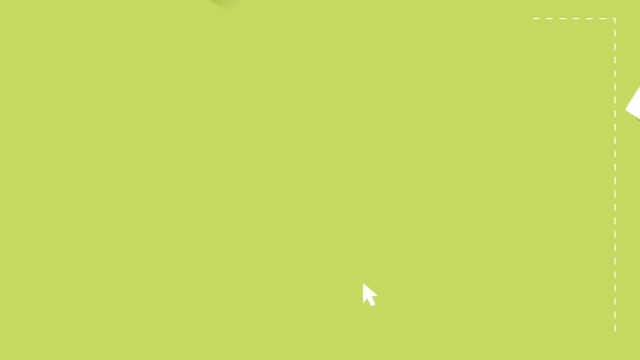 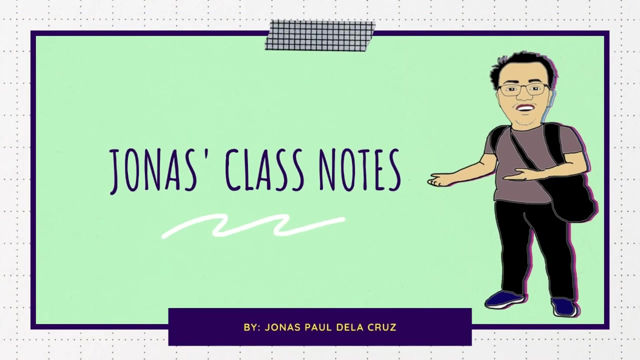 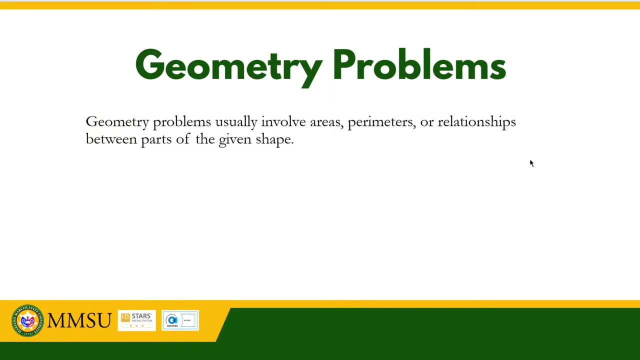 Hello everybody and welcome to another episode of our discussion on pre-calculus. We are still talking about the application of linear equation in one variable, We are done with the number problems and for this video we are going to talk about geometry problems, and geometry problems usually involve areas, perimeters or relationships. 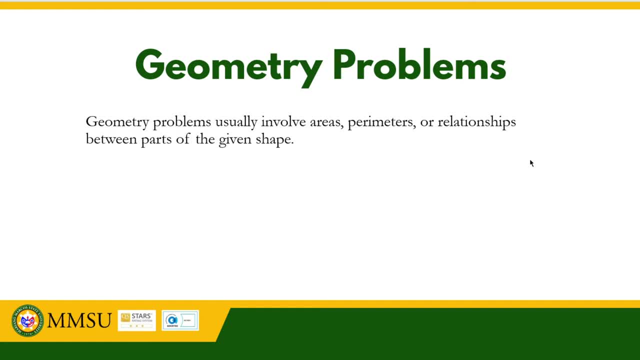 between parts of the given shape. So we will be talking or computing or solving two problems for this video, One for rectangle and one for triangle. But of course, geometry problems are not limited to just rectangle or triangle. You should have basic understanding of all the common shapes used in geometry, such as squares, the properties, 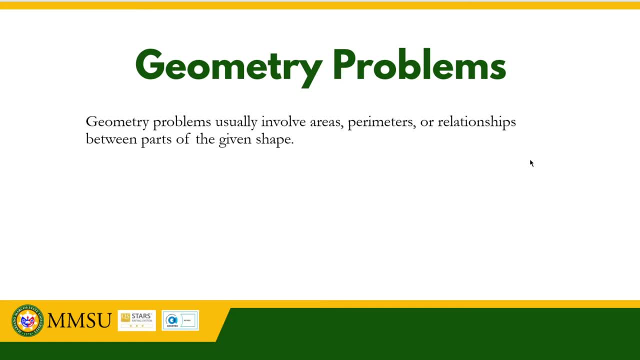 of a right triangle, a circle and the like. Okay, so before we proceed to our first example, do not forget to like this video and subscribe to my channel. Okay, so let us go to our first example. If a rectangle has a length that, 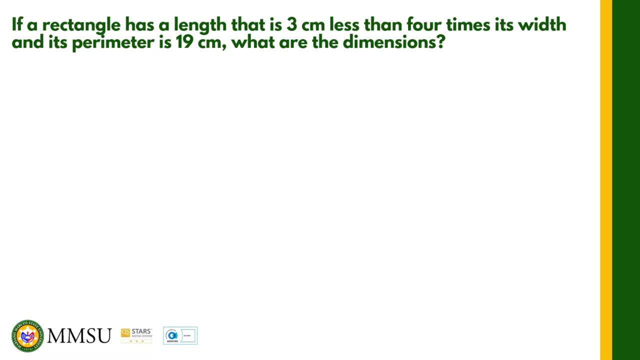 is 3 centimeters, less than 4 times its width, and its perimeter is 19 centimeters. what are the dimensions? Okay, just like in the previous examples on the number problems, we are given statements here, Two statements to be exact, And it's asking. 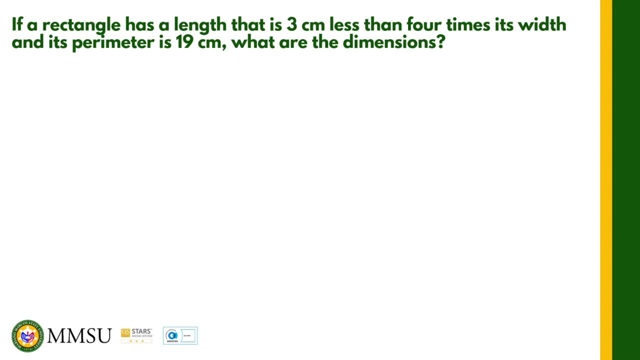 for the dimensions of the rectangle. Okay, so, before we proceed with the solution, it's very common that we need to draw the figure. Okay, so we are given a rectangle. So a rectangle is a four-sided polygon, right Two pairs of parallel sides, two pairs of parallel and. 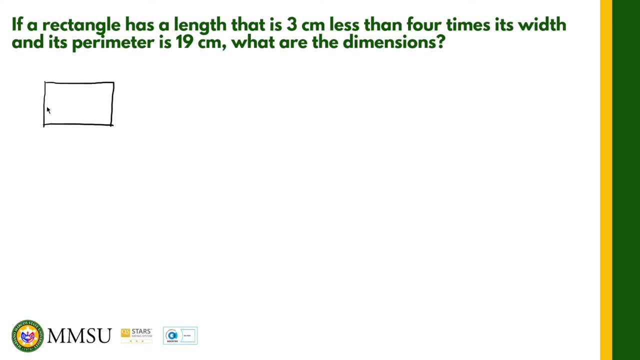 two pairs of horizontal sides And the two pairs of horizontal sides. Now, if the length of the rectangle is 7 centimeters, the length of the rectangle is 11 centimeters. The length of the rectangle is 1 centimeter. Okay, So we need to make sure that the length is equal. 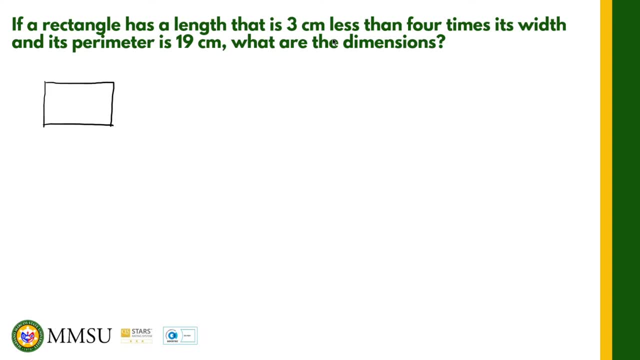 to the width. The length is 4 centimeters. Okay, The length is not equal to the width. okay, The length is not equal to the width. You should not make a mistake. Okay, so let's yung statement na yun is: 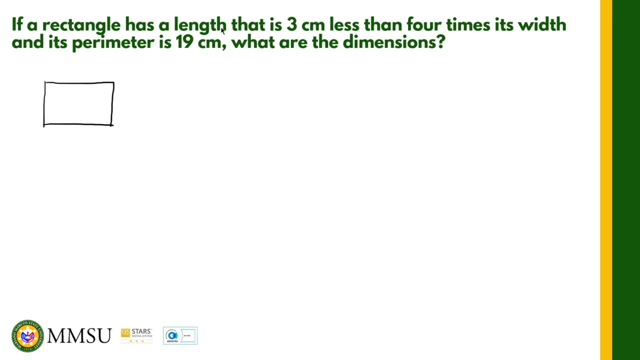 parang ini-equate: yung length in terms of width, ang i-let x, natin yung width. okay, so our representation for our variable will be: so let x be equal to the be the width of the rectangle. okay, and based from the first statement. 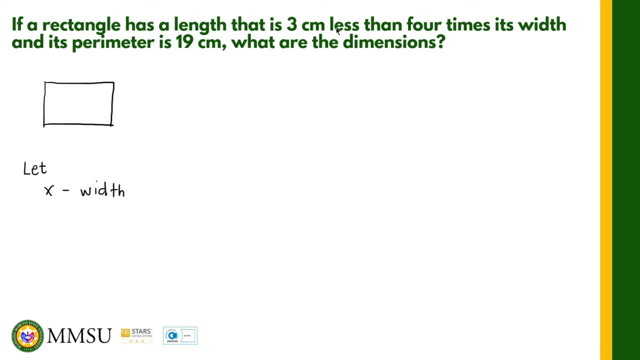 we are going to come up with a mathematical expression as our denotion for the length of the rectangle. okay, so the length is 3 cm less than 4 times its width, so 4 times the width minus 3, right, so that's 4x. 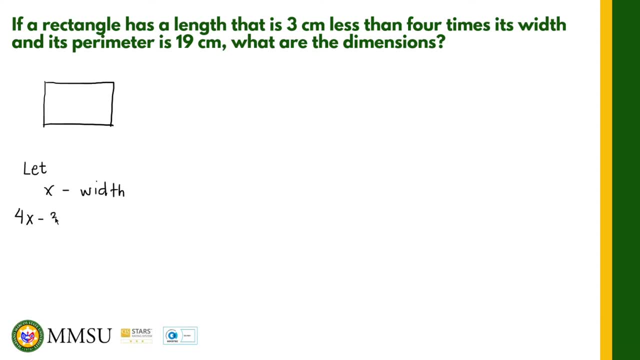 4x minus 3, so this is the length of the rectangle. so if this is the length, right, that is the length. this is the width, okay? so the perimeter of the rectangle is just equal to twice the length plus twice the width. that's the sum of all the. 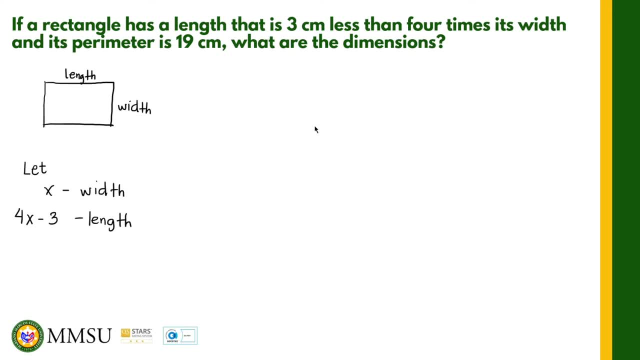 sides of the rectangle. okay, so equating it to 19 cm, because the given perimeter is 19 cm, that's dalawang width, that's x plus x or 2x, and then dalawang length, so that's 4x minus 3. 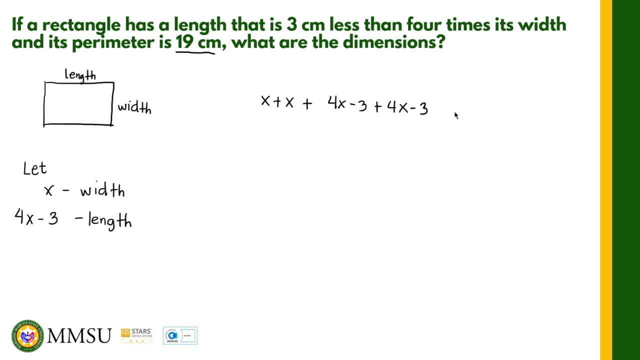 plus another 4x minus 3, and the perimeter is equal to 19 cm. okay, all units in cm. and then we perform the algebraic operations for this one to solve for x. so we have x plus x plus 4x plus 4x. 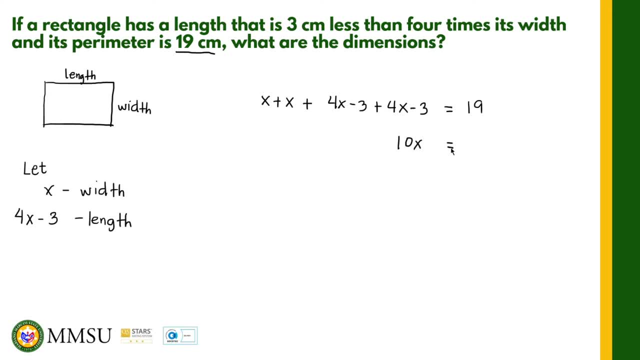 that's 10x okay and equal. this is equal to 19. we have minus 3 and minus 3 on the left side of the equation. if we transpose this to the right side of the equation, becomes plus 6. so 19 plus 6 is. 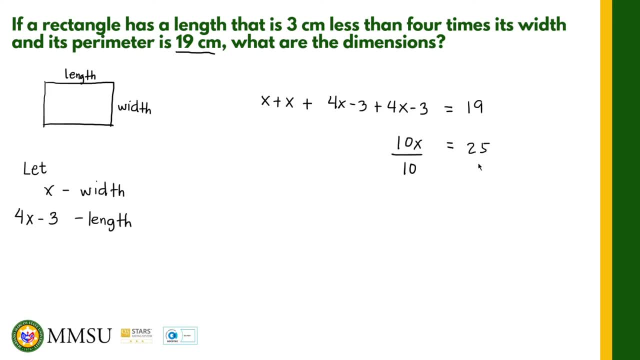 25, and then we divide both sides by 10, divide both sides by 10. therefore, x is equal to 2.5 cm. okay, now that is the width of the rectangle. so to solve for the length, we have 4x minus 3. 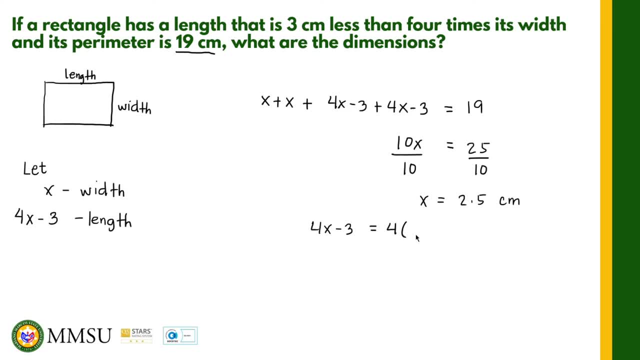 okay, so 4x minus 3 is equal to 2.5 cm. okay, so 4x minus 3 is equal to 2.5 cm. okay, so 4x minus 3 is equal to 2.5 cm. 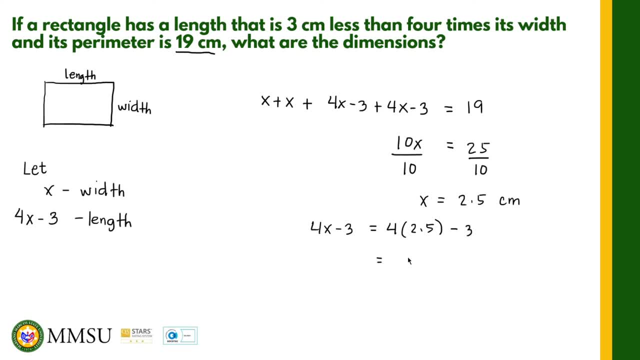 minus 3. okay, so 4x 2.5 is equal to 10, 10 minus 3, so that's 7 cm. okay. so to answer the problem: what are the dimensions? so the dimensions: okay, we can write: the length is equal to 7 cm. 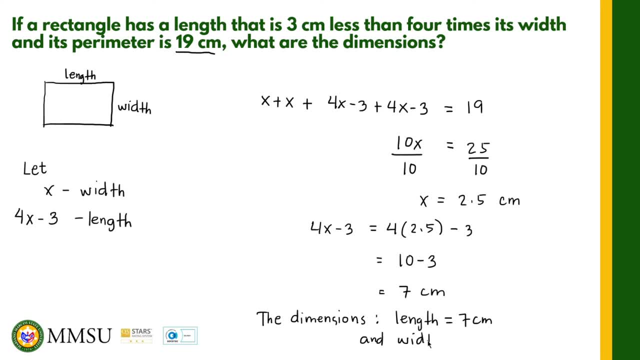 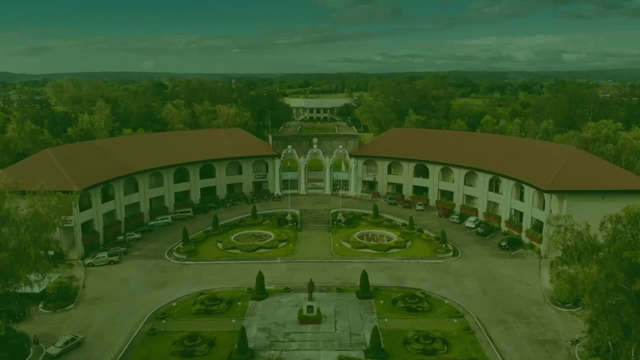 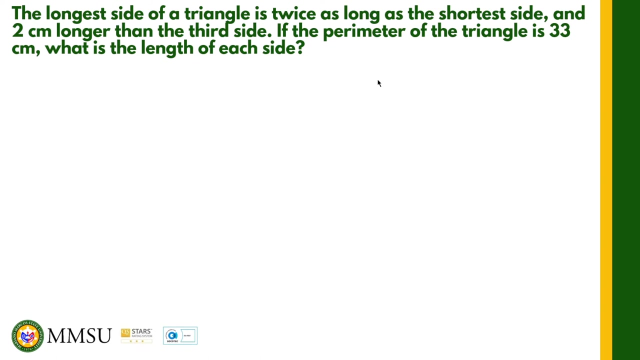 and width equals 2.5 cm. okay, so that's our conclusion. so that answers the problem for this example. so let us answer one more problem involving geometry. so for this example, we are going to talk about a triangle. okay, so the longest side of a triangle. 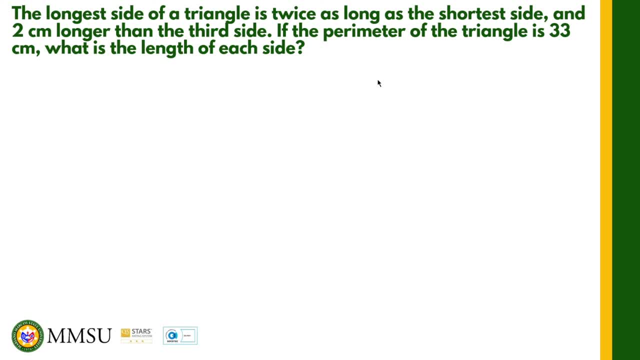 is twice as long as the shortest side and 2 cm longer than the third side. if the perimeter of the triangle is 33 cm, what is the length of each side? okay, so we know that a triangle is a three-sided figure, right? 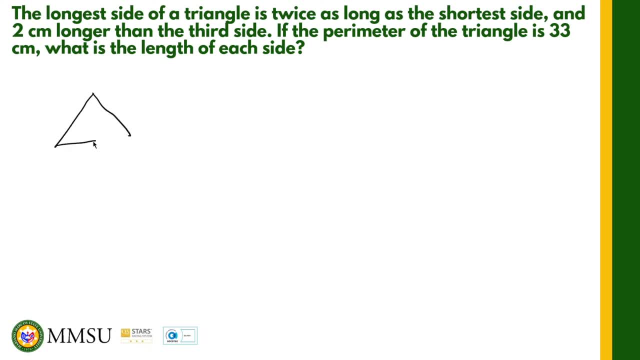 a three-sided polygon. okay, something like this. okay, so the first statement says that the longest side of a triangle is twice as long as the shortest side. so that's a relationship between the longest side and the shortest side. so we can actually write our representation here. 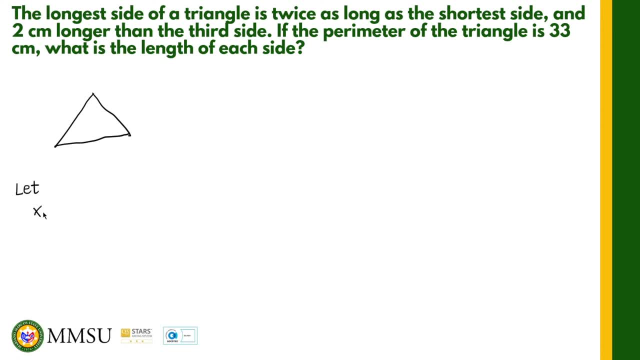 so we let x. okay. it's up to you what you want. you can represent the longest side or the shortest side as x. okay, but for this example, I'm going to represent x as the shortest side. shortest side- okay. and the first statement says that the longest side of a triangle is twice as long as the shortest side. 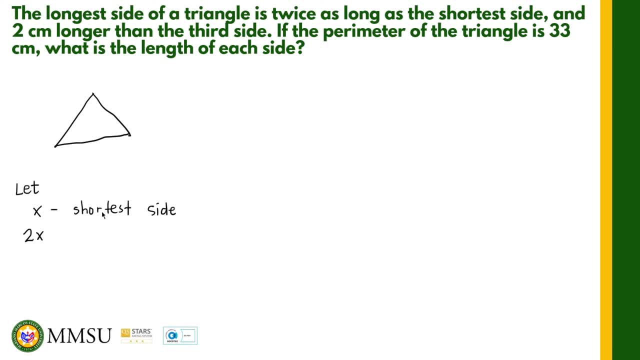 therefore, that's 2x twice. the shortest side is 2x. this is the longest longest side. okay, how about the third side? okay, so the second statement says that the longest side of the triangle is also 2 cm longer than the third side. this means: 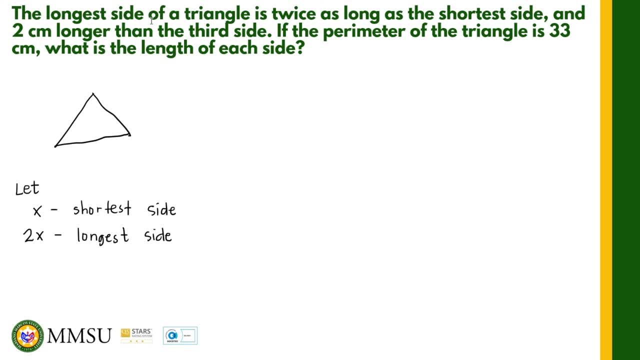 that the third side is 2 cm shorter than the longest side, right? so if the longest side is 2x and we know that the third side is 2 cm shorter than the longest side, therefore we can represent the third side as longest side: 2x. 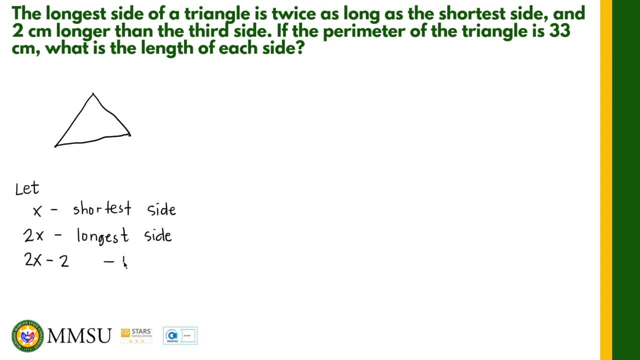 minus 2. okay, this is the third side. so now, we now have our representation for the three sides of the triangle. so we have x- 2x and 2x minus 2. okay, then what is our equation? let us look at the next statement here: the perimeter of the triangle. 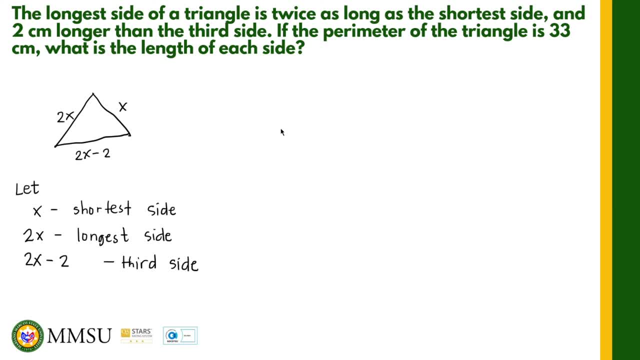 is 33 cm. that means if we add all the sides of the triangle we will get 33. so that's: if x, 2x plus 2x minus 2, the third side is equal to 33. okay, so we combine like terms, that's. 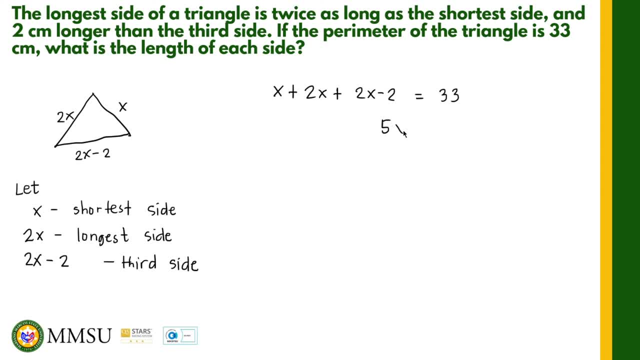 x plus 2x plus 2x, that is 5 x. okay, so 33 plus 2. transpose minus 2 to the right side, that's 35, and then we divide both sides by 5. therefore, x is equal to x is equal to 7.